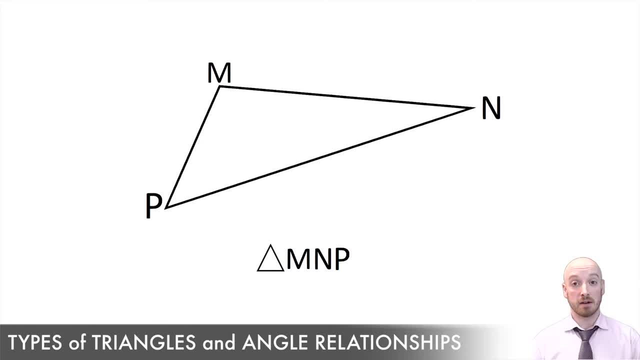 if we're going to be labeling the side lengths, they get the exact same letters as those angles get, but in lowercase instead of uppercase. So the side lengths in triangle MNP are also going to be called M, N and P, but in lowercase. And when we label those sides it's really important that you. 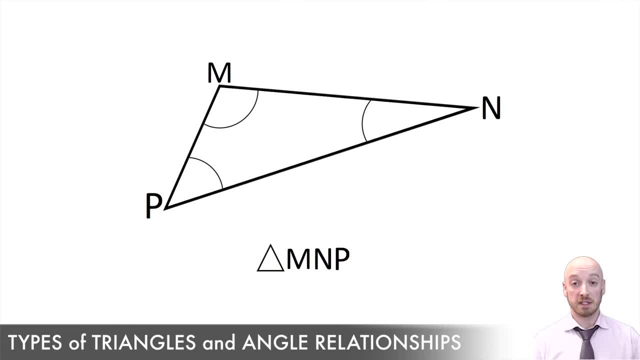 label the side lengths across from the angles with the exact same letter, just in lowercase. So side M is across from angle M, side N is across from angle N and side P is across from angle P, Although the side lengths are in lowercase. Now, remember I mentioned the types of triangles that 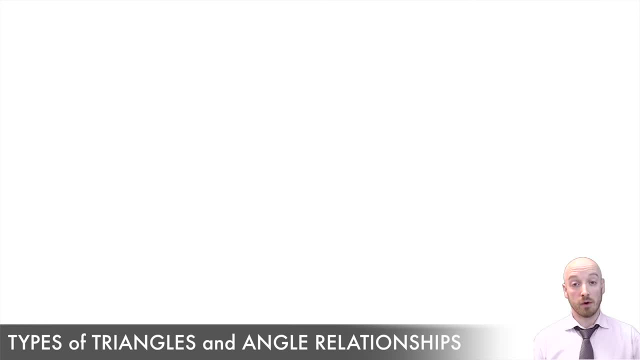 we're familiar with. Well, the types of triangles that we've learned before are called equilateral, isosceles and scalene. Here's what you need to know about naming those triangles in that way, Equilateral triangles have three side lengths that are the exact same, and they also have three angles. 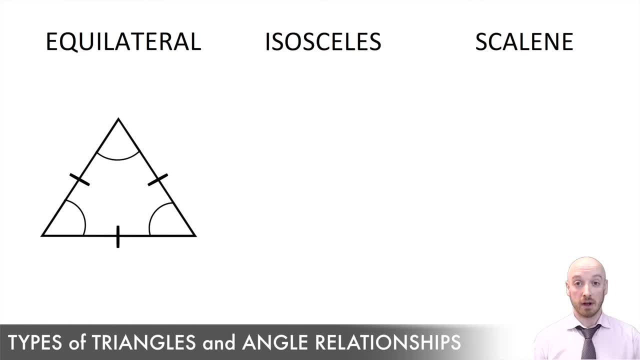 that are the exact same And those three angles in an equilateral triangle are all 60 degrees. Remember those three identical angles still have to add up to 180.. The next type of triangle that we've probably heard of before is called isosceles. An isosceles triangle has two side lengths that are identical in 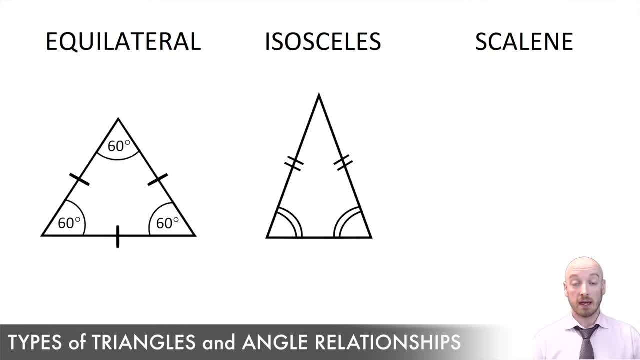 length and then two angles that are identical also, And a scalene triangle is just a triangle that has three different side lengths with three different angles on the inside. So that's how we name triangles: based on their side lengths, but we can also name triangles based on the types of angles that are in them. So 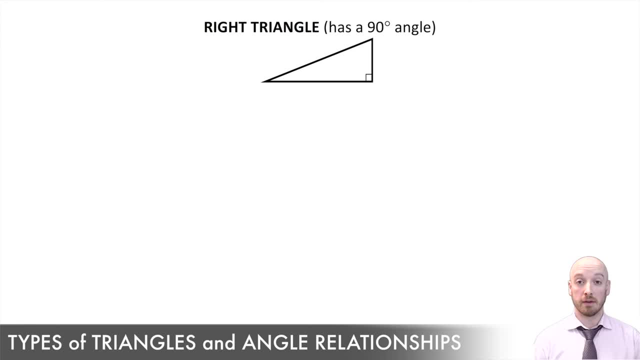 we've talked about right triangles before. A right triangle is a triangle that contains one 90 degree angle in it, And in the non-right triangle category we have acute triangles and obtuse triangles. Acute have three angles that are each less than 90 degrees, and an obtuse triangle has one angle, that's. 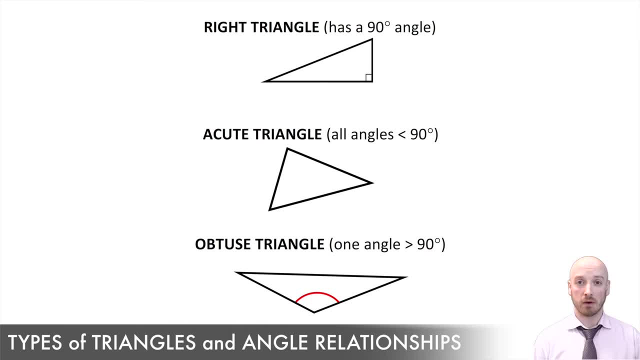 bigger than 90 degrees. The other two obviously have less than 90 degrees And in the non-right triangle category we have to be smaller than 90.. Now, speaking of angles, we're going to have to learn a little something about angle relationships also, and you're going to have to pay close attention here. 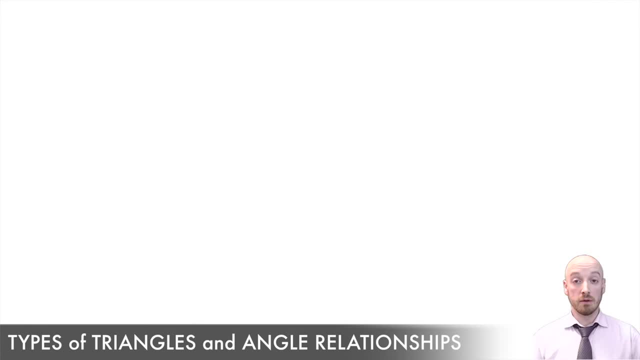 Now let me start explaining angle relationships by pointing out two that you've probably learned before. Complementary and supplementary angles are angles that either add up to 90 degrees if they're complementary, and supplementary angles, when put together, are going to form a perfectly straight line. Any angles that get together to form a straight line add up to 180. 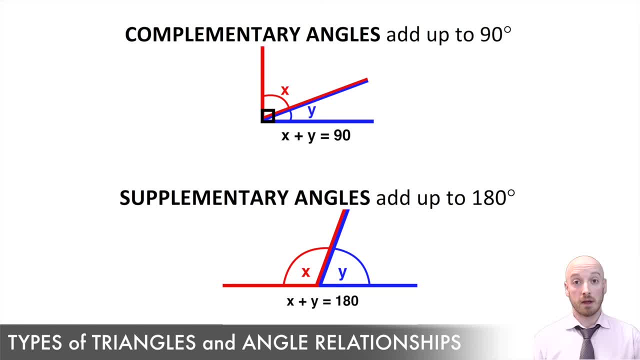 degrees. Now, usually it's just two angles that are either complementary or supplementary, but it could be any number of angles that, when put together, make a 90 degree angle if they're complementary and that make 180 degrees if they're supplementary. Now here's where things. 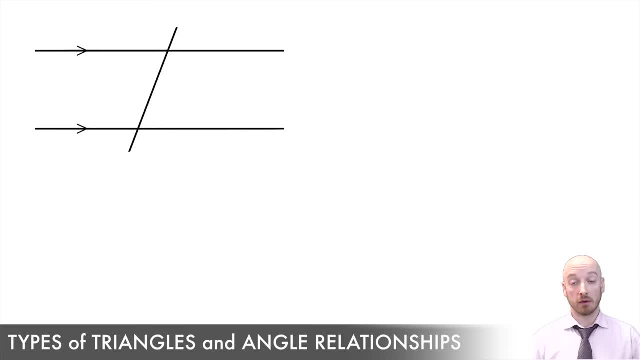 are going to get a little bit complicated. Take a look at the screen here. What you're looking at are two parallel lines with one straight line that's passing through both of them. That straight line that passes through the parallels is called a transversal line, and it forms a whole bunch of. 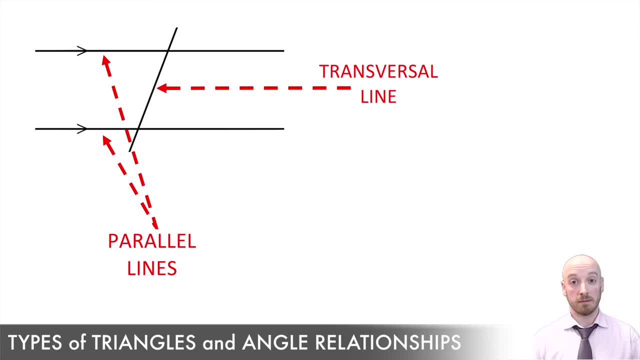 angles that are complementary or supplementary. Now the problem is that when you're looking at angle relationships that I'll explain to you right now. First let me just point out the angles to you that are supplementary here. Remember any two angles that form a straight line. 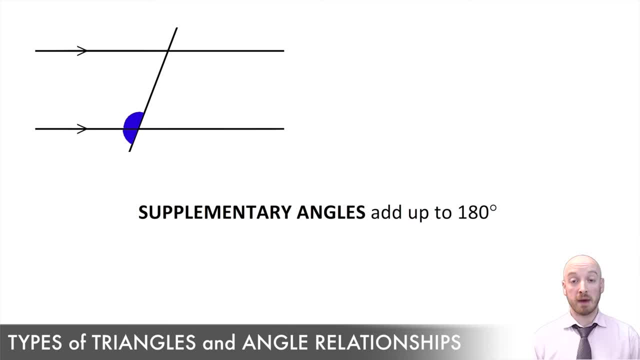 are called supplementary angles. So here, when we have two angles back to back, no matter how that straight line is formed, whether it's on the parallel or on the transversal, we have supplementary angles. So what's handy about supplementary angles? 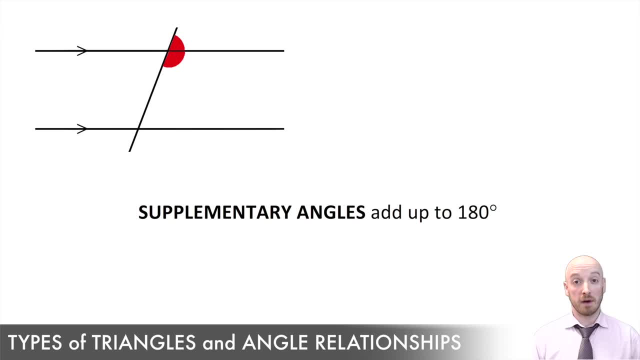 Well, if you're given the measurement of one of those supplementary angles, you can find the measure of the other angle by just subtracting the first one from 180.. Now we have a new concept here, and it's something called vertically opposite angles. 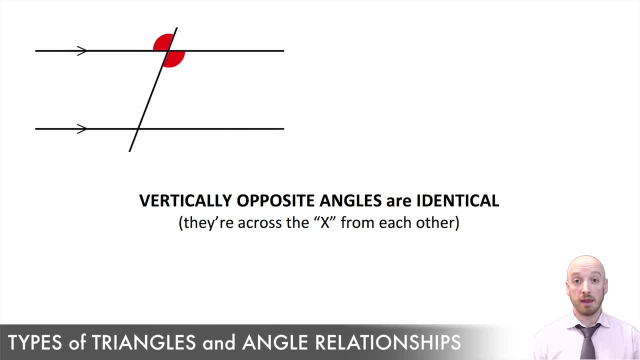 Vertically opposite angles are the exact same as each other and they exist right across from two intersecting lines. Notice how any two straight lines form sort of an X shape where they cross. What's important to know is those vertically opposite angles are identical to each other. 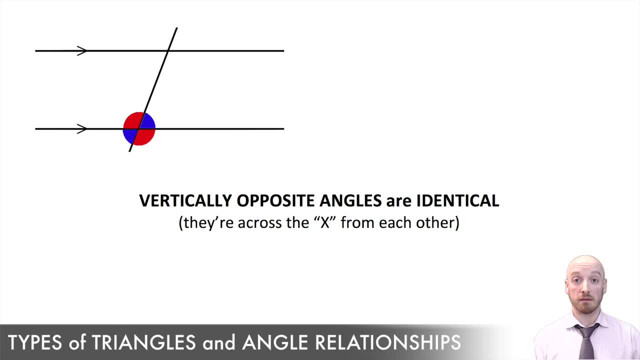 So if you know the measure of one of them, you can take it and use it as the measure of the other. Up next is what we will call alternate interior angles. So these angles are on the opposite sides of the transversal line and on the interior. 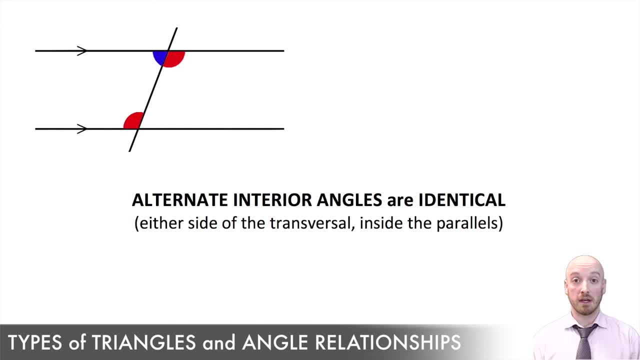 of those parallel lines. That's why we call them alternate interior angles. And what do we know about alternate interior angles? Well, it might be obvious from what you see on the screen here, but they're identical also, So anytime we have two angles that are on alternate sides. 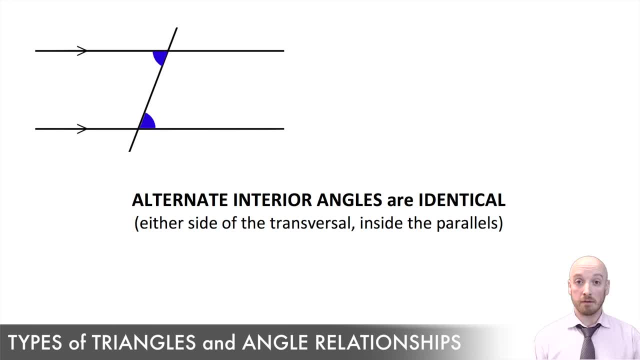 of that transversal line on the interior of the parallels. those are identical angles also. Now, up next, we have something called alternate exterior angles. Think of everything we just said about alternate interior, but apply it to the outside of the parallels.